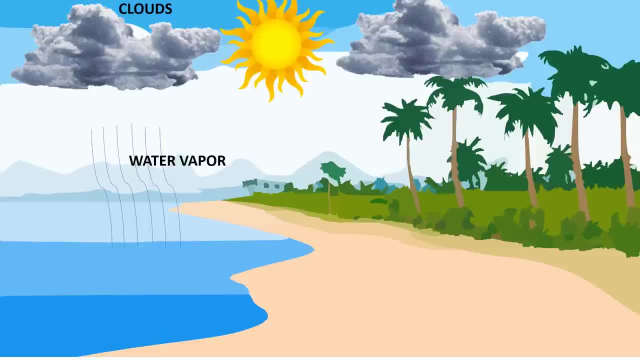 In the same way, the water vapors from the hot sea or rivers moves up the sky and cools down to form clouds. This process in which a gas changes to solid is called evaporation. The process in which a gas changes to liquid is known as condensation. 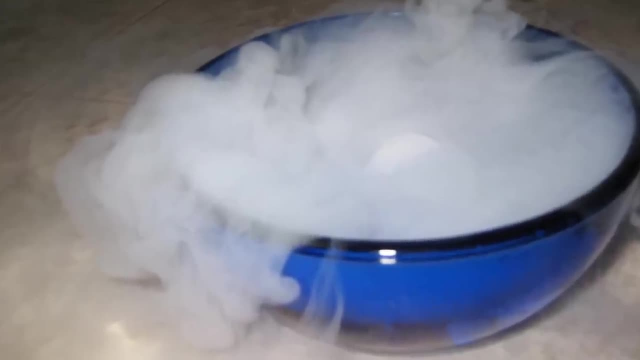 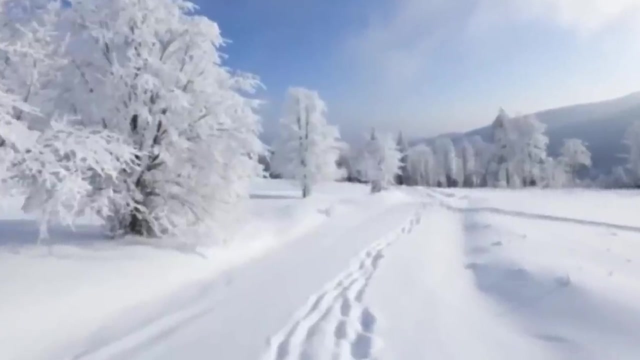 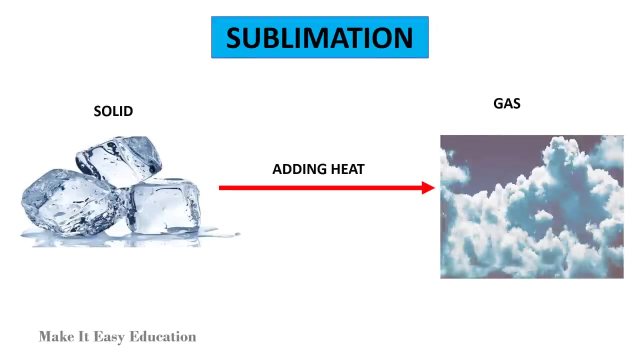 Dry ice change into gas directly without changing to liquid. Snow can also change into gas directly in the winter months without melting. The process in which solids directly change to gases is known as sublimation. Deposition is the reverse of sublimation. 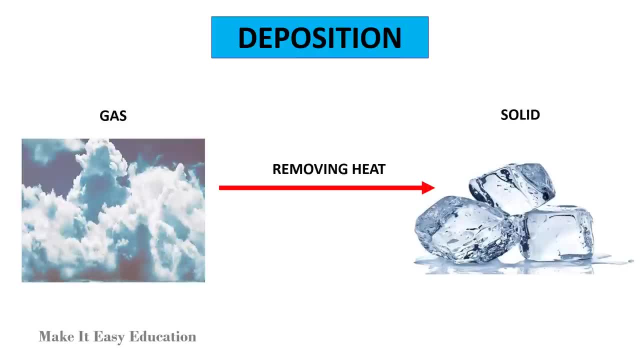 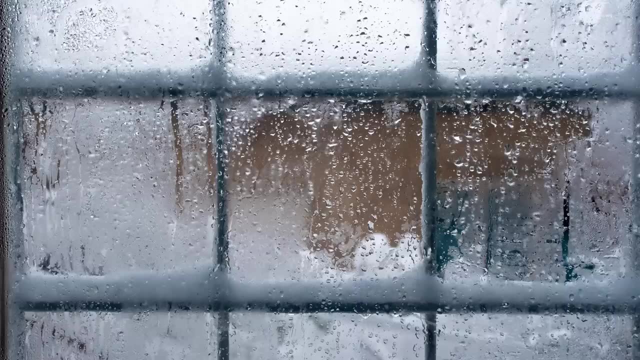 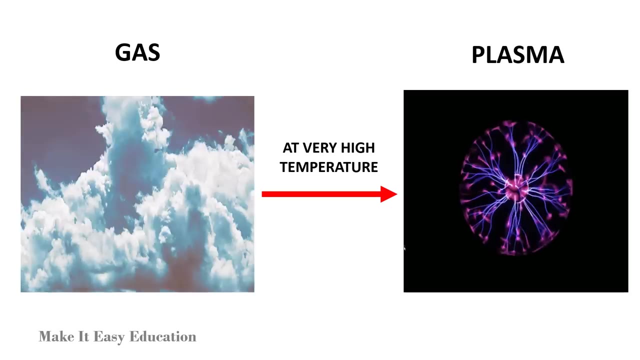 In this process the gas changes into solid directly, without passing through the liquid. It is how snow forms in clouds and how frost form on the windows. Another state of matter called plasma occurs when the gas is heated at very high temperatures. The sun is mostly made of plasma. 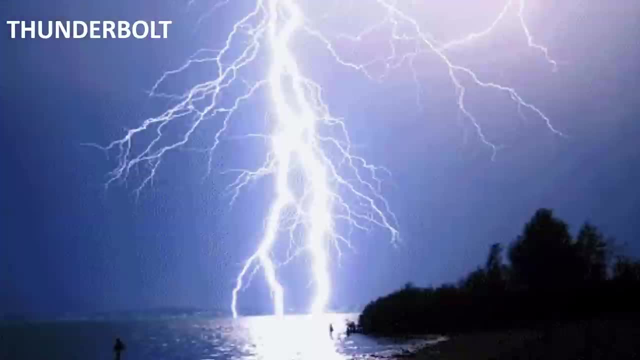 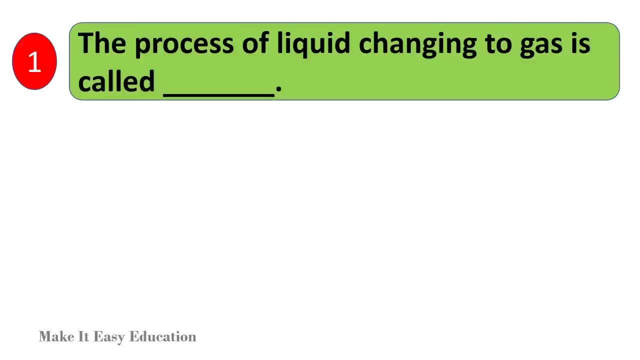 Lightning or thunderbolts makes plasma Question Time. At the end of the day, is it possible to change to plasma? Does light come from the sun? How can light change from the sun? What can the sun do? How can light change from the sun? 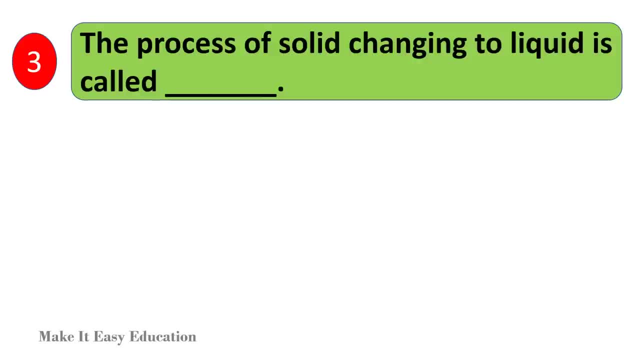 How does light change from the sun? How can light change form? the sun, How can it change from the sun to the sun? How does the light change from the sun to the sun? What is the property of light, or what part of light does it move into? 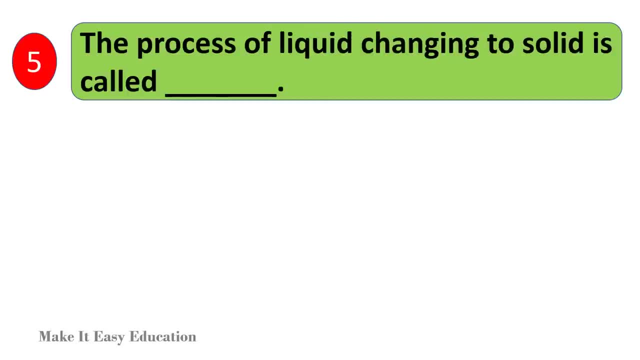 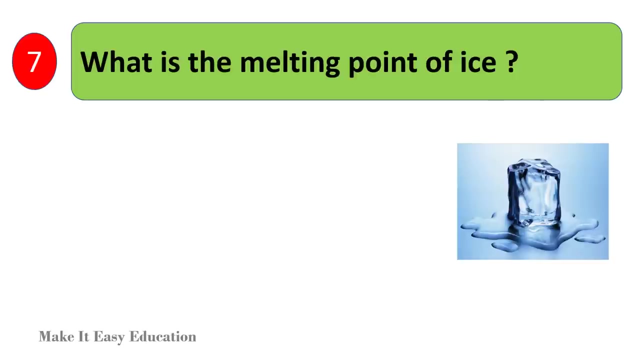 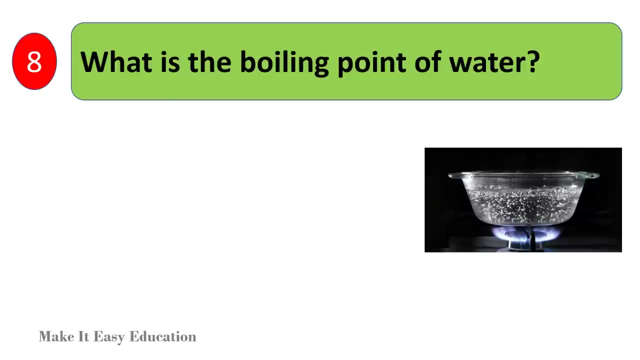 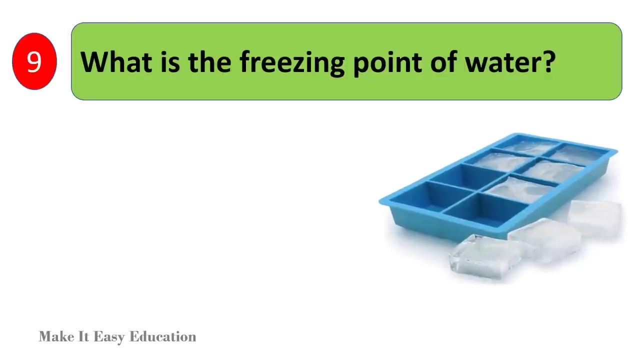 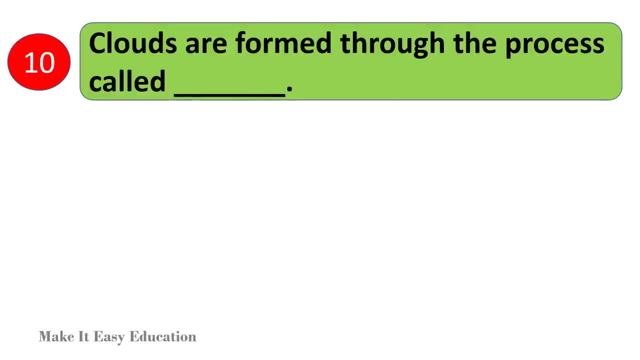 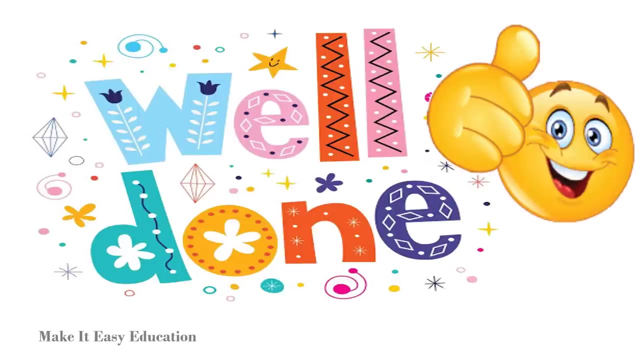 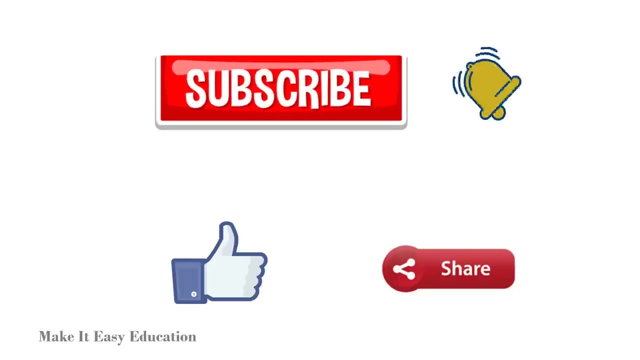 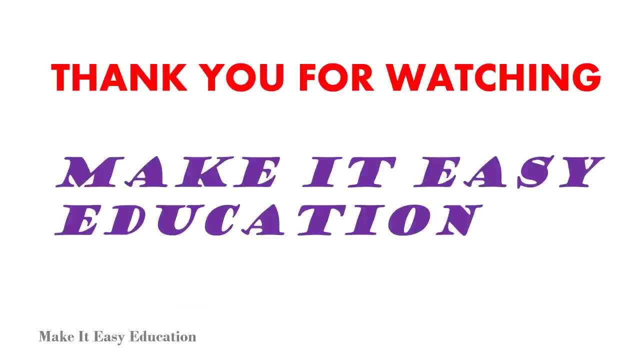 Also, is this energy running in the earth or does light occur through it? Thank you, Thank you. Click the notification bell. Thank you for watching. Make It Easy Education.